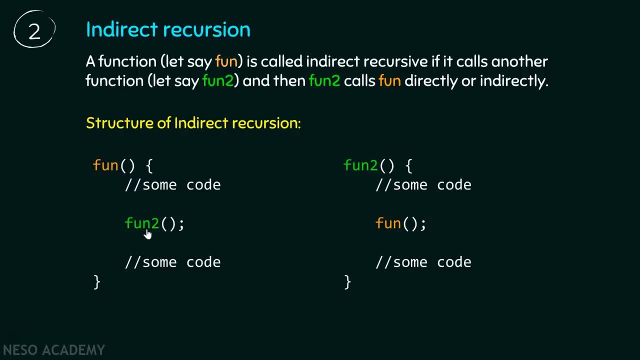 and inside this function you are not calling this function, but you are calling another function, let's say fun2, whose definition is available over here. And inside this function you are calling fun function. If you observe this code structure carefully, you are calling function fun, only right. 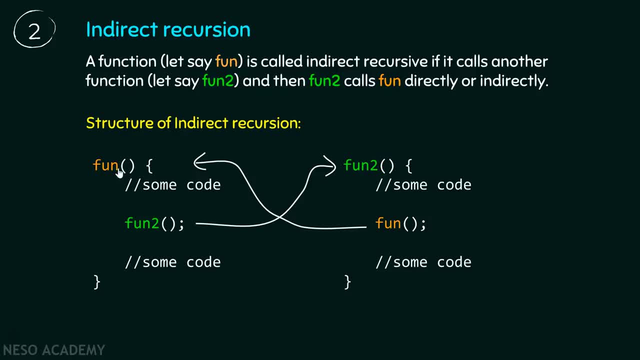 This is a recursion, for sure, But you are calling this function indirectly, Right? You are first calling fun2 and then, from fun2, you are calling fun function. This is called indirect recursion. Okay, Let me repeat the definition for you: A function, let's say fun. 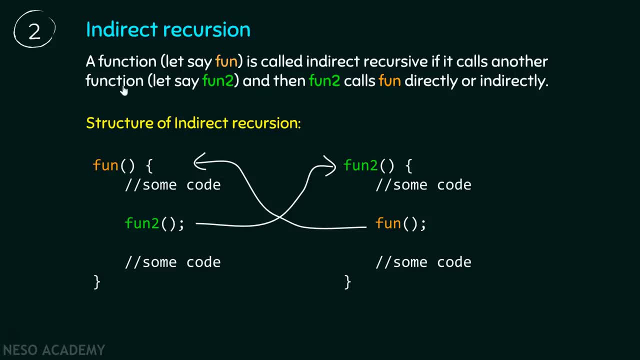 is called indirect recursive if it calls another function, let's say fun2.. And then fun2 calls fun, directly or indirectly. Right, I know it will be little bit difficult for you to understand the concept behind indirect recursion, And you want to know where. 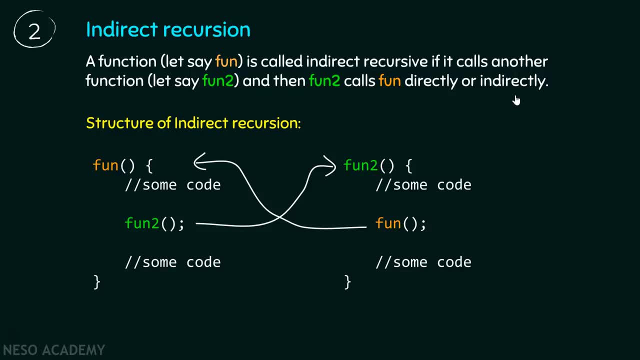 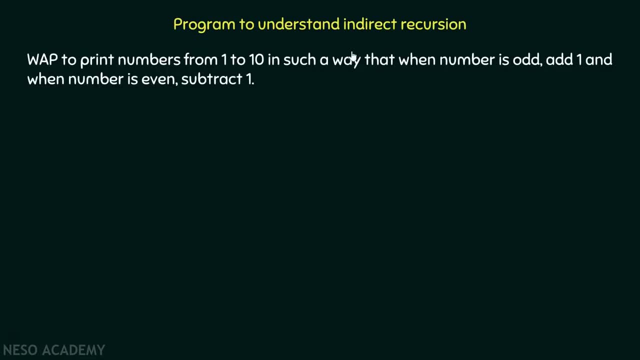 indirect recursion is useful. So, to address all these doubts, let me give you one program which will help you to understand indirect recursion in better details. Write a program. This is the short form of writing. Write a program. Write a program to print numbers from one to ten. 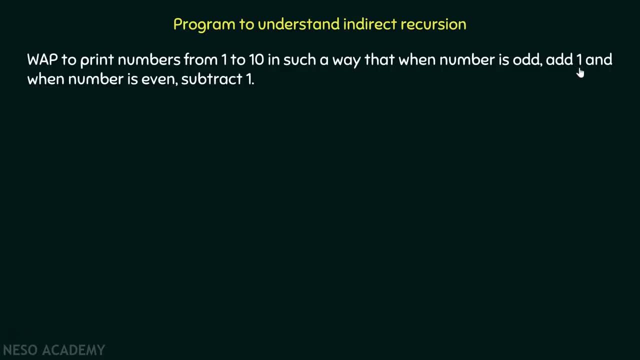 in such a way that, when number is odd, add one, And when number is even subtract, one. You want this program to produce an output something like this: When you encounter an odd number, you should add one to it, And when you encounter an even number, 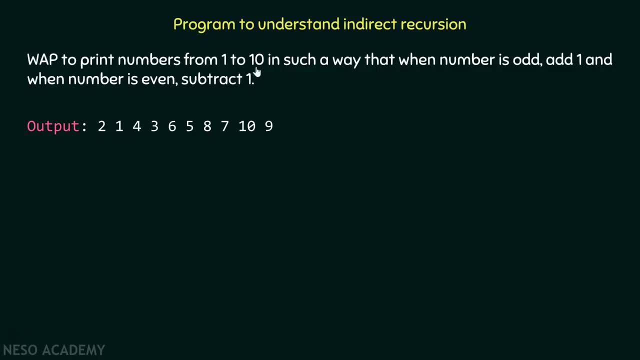 you should subtract one from it. That's what we have to do, right? And we have numbers from one to ten. As we have numbers from one to ten, we should add two, because the number one is odd. right After that, you encounter number two. 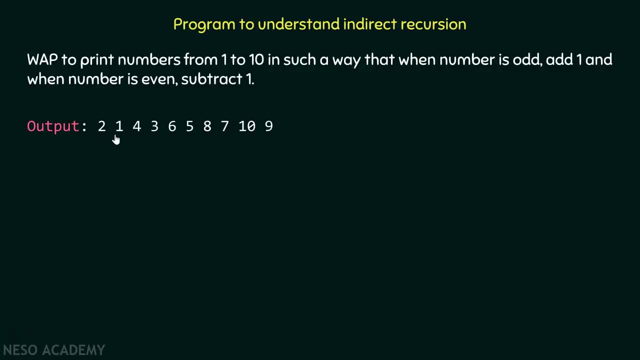 As number two is even, therefore we need to subtract one from it, So it becomes one right. And then after that we encounter three. As three is an odd number, we have to add one to it, So it becomes four. 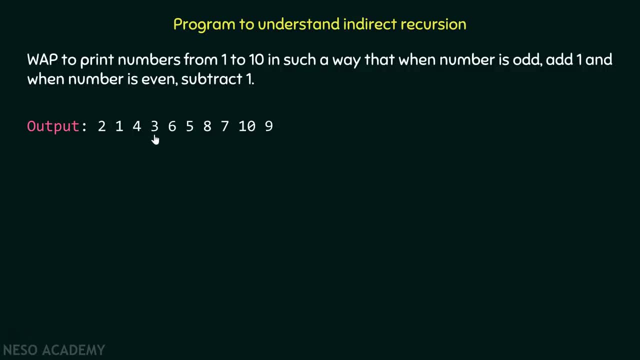 And then we encounter number four, which is an even number, So we should subtract one from it, So it becomes three, And then we can code this particular program to produce an output something like this: Suppose we have two functions: odd and even. 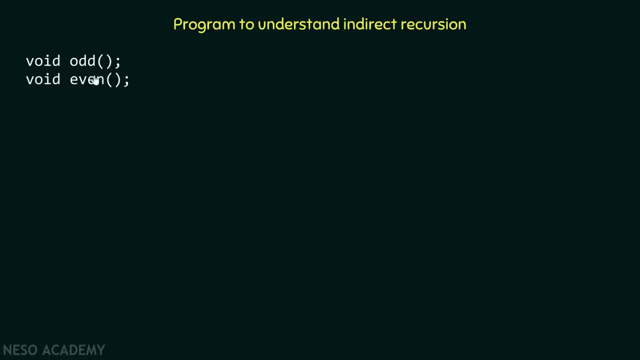 As the name itself suggests, odd function will handle odd numbers and even function will handle even numbers. Whenever an odd number is encountered, it will add one to it and print it on the screen, And when an even number is encountered, it will subtract one from it. 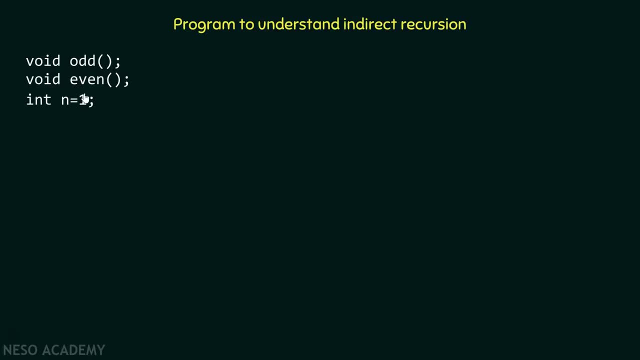 and print it on the screen And suppose we have one variable n. basically this variable n depicts numbers from one to ten. Now here is the definition of the function odd. Inside this function we have an if construct and then immediately after that we have return statement. 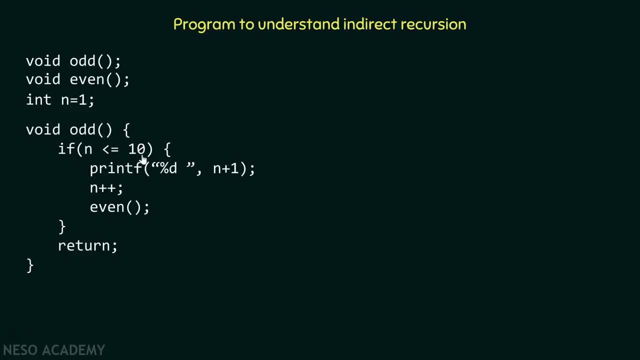 What does this? if construct say: If n is less than or equals to ten, then you will print n plus one on the screen, As odd function is going to handle odd numbers. so if suppose we encounter number one, so it will print two on the screen. 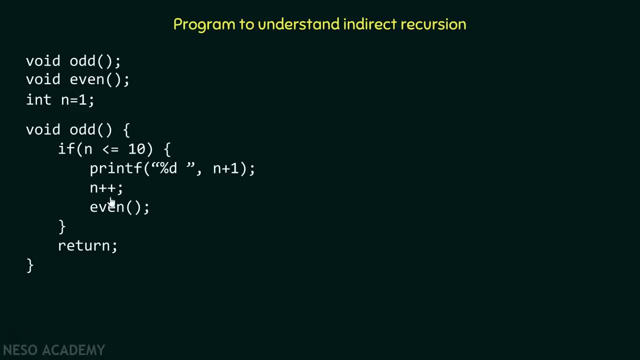 Right. And after that we increment the value of n so that it becomes an even number, so that we can handle that number Right. And here is the definition of even function as well. The code of even function is exactly the same as the odd function. 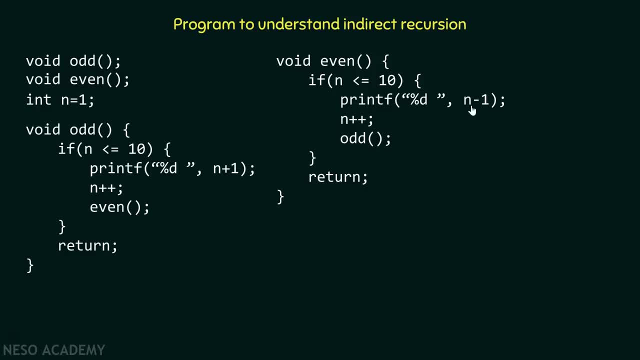 but there is one difference you can encounter over here: Instead of n plus one, you have n minus one. After this function, we have a main function and inside this main function we are calling odd function. Why we are calling odd function? Because the first number we encounter is one. 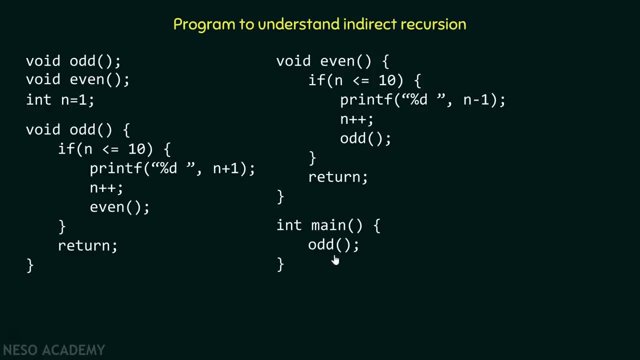 and it is an odd number. Therefore, we first have to call the odd function in order to handle that number. This is the output we are expecting: 2, 1, 4,, 3, 6,, 5,, 8,, 7,, 10,, 9.. 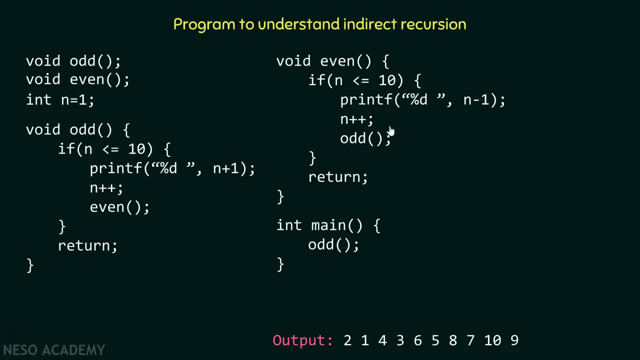 And now let me simulate this code with the help of stack. This is what we are doing usually when we see recursive programs. Suppose we have a stack like this and initially, as we know, main function is called. Inside this stack, the activation record of main function will be created. 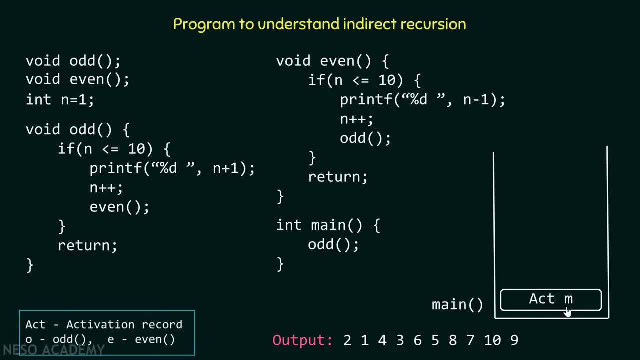 Right, Which is denoted by act. Act simply means activation record. O means odd function. Whenever you find a symbol O, you should replace this with odd function, And whenever you find the symbol E, you should replace this with even function. Okay, M means main. 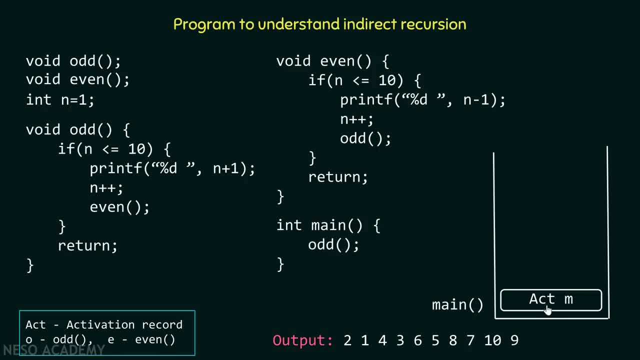 and act means activation record. So basically, what does it mean is you are storing the activation record of this main function inside this stack. Okay Now, as inside this main function, you are calling the odd function. Therefore the control terminal transfers to the odd function. 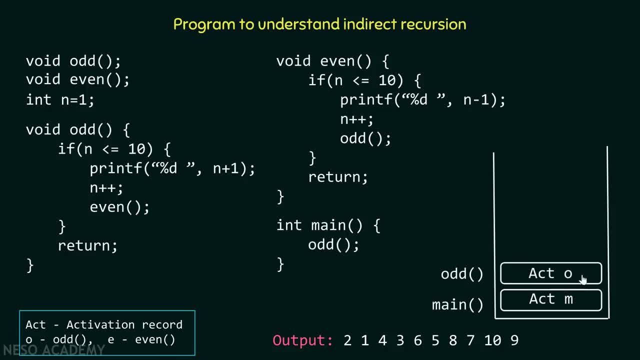 And the activation record of the odd function will get stored inside the stack, As we have called the odd function, and inside this odd function, as you can see, we have an if construct where we are checking this condition is n less than or equals to 10.. 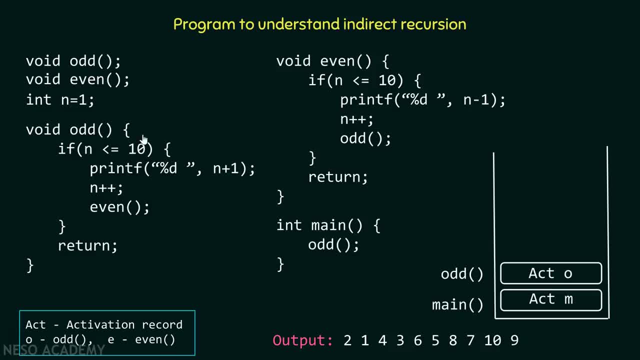 As n is initially 1 and 1 is less than 10, it is satisfied. Therefore we come inside this if construct and we simply print value 2 on the screen Right And then after that we increment the value of n so that n becomes. 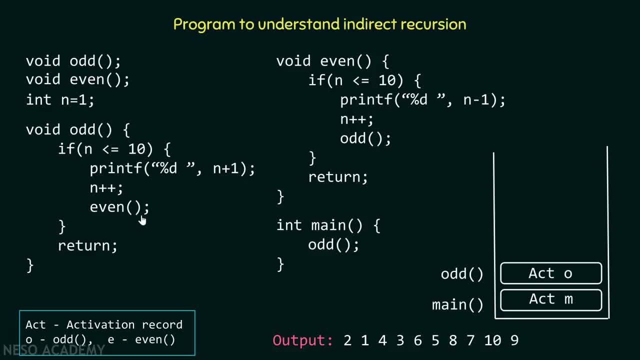 2, and now we simply call even function. This means now the control transfers from odd function to even function and the activation record of even function will get stored inside the stack. Now, inside this even function, again we encountered this: if construct as n is again less than 10, 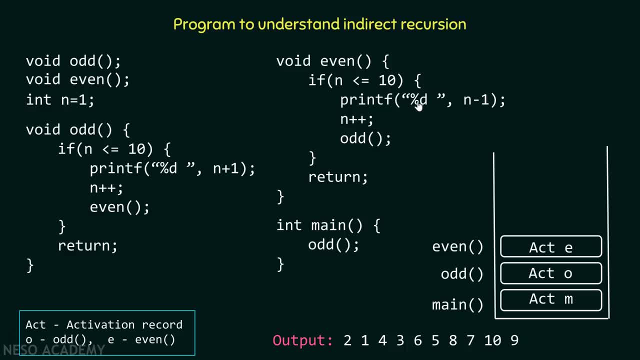 because n is equal to 2 and 2 is less than 10.. We go inside this. if construct, we simply print value 1 on the screen, because 2 minus 1 is 1.. Right, And then after that we increment the value of n. 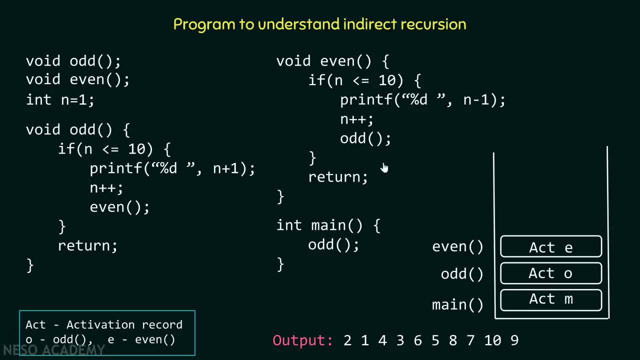 3 and then again we call odd function. Now control will again transfer to the odd function and the activation record of odd function will be created inside the stack. As value is 3 and 3 is less than 10, again, condition is satisfied. 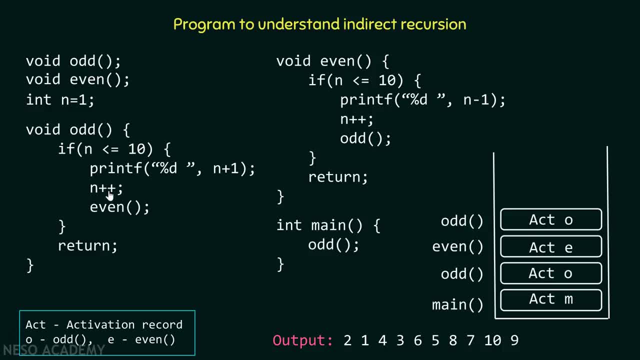 We simply print value 4 on the screen and then we increment the value of n. Now n becomes 4 and we simply call even function. Now the control transfers from odd function to even function and the activation record of even function is maintained inside the stack. 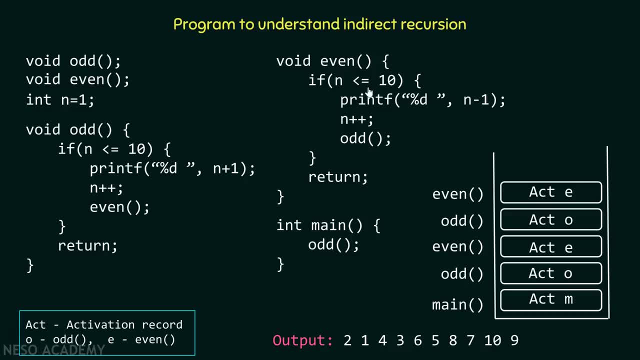 As n is equal to 4 and 4 is less than 10, condition is satisfied, We come inside the if construct, and here we will simply print value 3, because 4 minus 1 is 3.. Right, And then after that you increment the value of n. 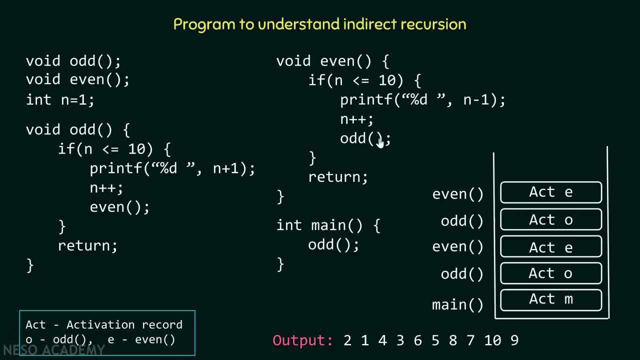 Now n becomes 5 and we again call the odd function, And the activation record of odd function is also maintained inside the stack Right Now, when n is equal to 5, we print value 6 on the screen Right And then again value is incremented. 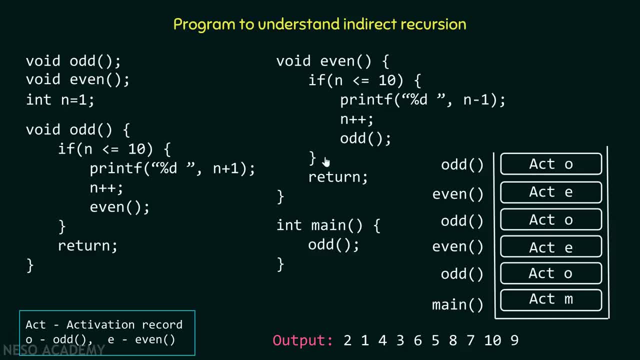 and even function is called. This process will continue like this way only until and unless we obtain n equals to 11.. When we encounter n equals to 11, the condition itself fails and we start returning. Right Now, suppose after this point we are returning? 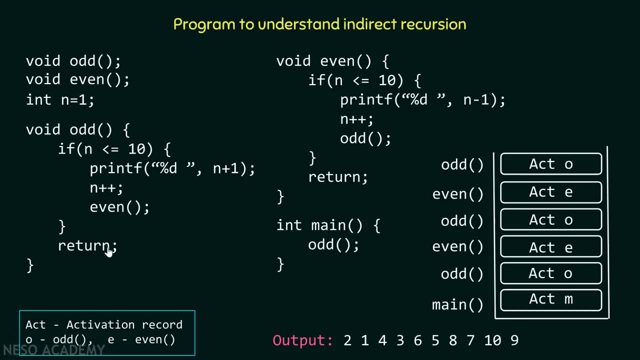 As return means you will return back to the position where you left off. As we are returning from the odd function, the activation record of odd function will get popped out of the stack, So we will return back to the even function where we left off at this point. 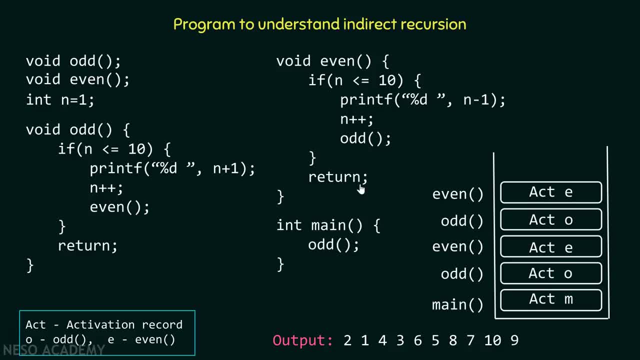 Right After this, there is nothing. You have encountered. return statement again. This means you will return back to the position where you left off, means you will return back to the odd function at this particular point And again after that you find return. This means you again return back. 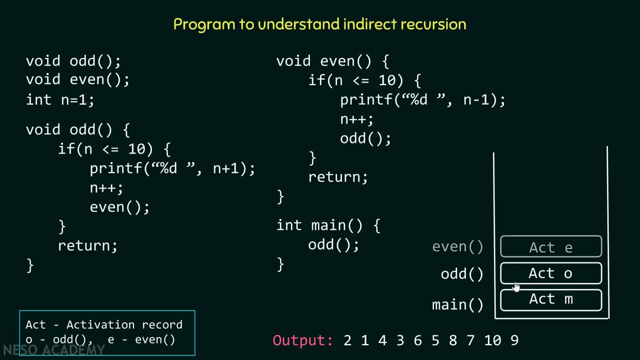 to the even function And, similarly, the procedure continues. You are simply returning back. Finally, you encountered the main function and, as you can see, at this point there is nothing written. This means this main function will simply pop out of the stack And the execution is completed. 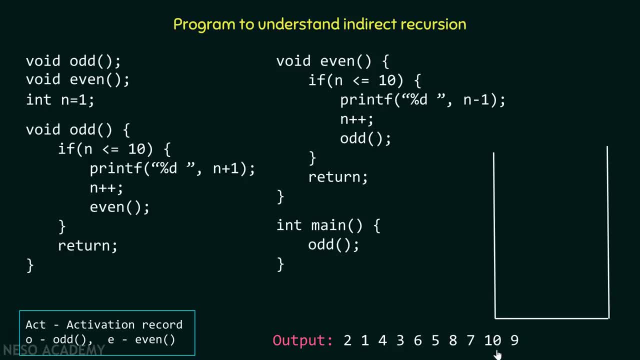 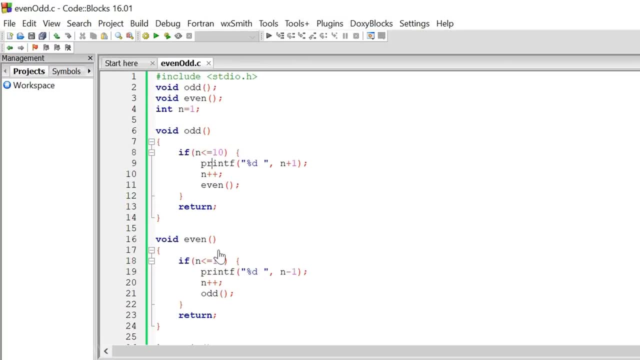 Now let me execute this code for you and check whether this output- whatever we are expecting- is what we are getting or not. Here is the code, which we have seen already. We have an odd function and an even function, and after that we have a main function. 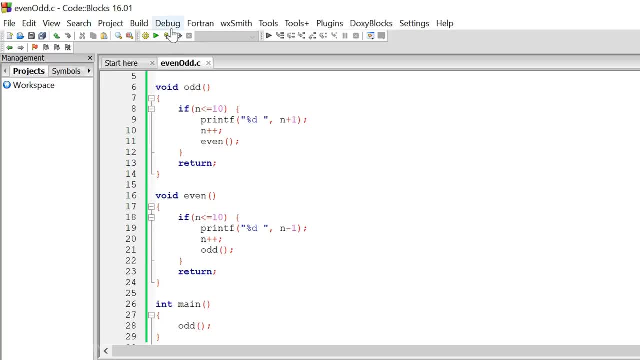 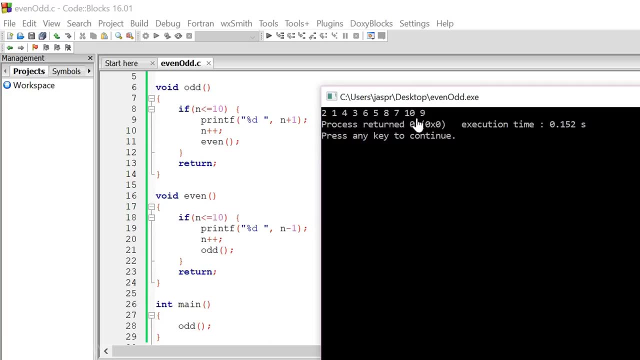 and here we are calling an odd function. Let's see whether this code works fine or not. Yes, it produces the output 2143658719, which is the expected output. Ok, friends, this is it for now. Thank you for watching this presentation.